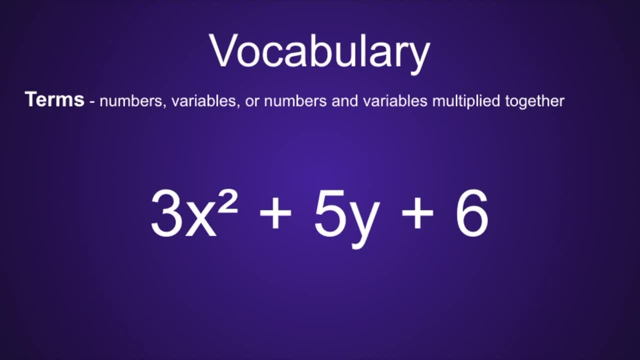 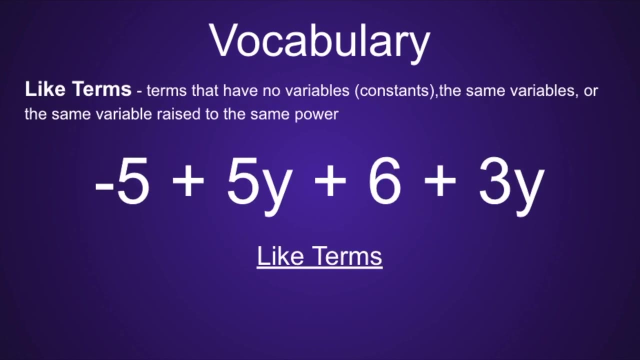 multiplied together. So in the expression 3x squared plus 5y plus 6, there are 3 terms: 3x squared, 5y and 6.. Now let's take a look at like terms. Like terms are terms that have no variables. These 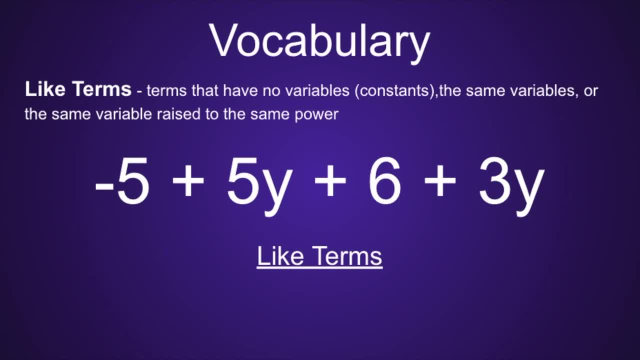 are called constants, The same variables or the same variable raised to the same power. In the expression negative 5 plus 5y plus 6 plus 3y, the like terms would be 5y and 3y because they both have the variable y and negative, 5 and positive 6.. 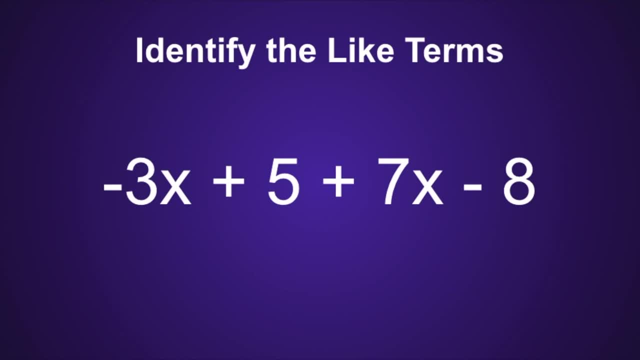 Now I want you to practice one In the expression negative: 3x plus 5 plus 7x minus 7x plus 8, I want you to determine the like terms. I recommend you pause the video now and then resume when you're ready to see if your like terms are correct. 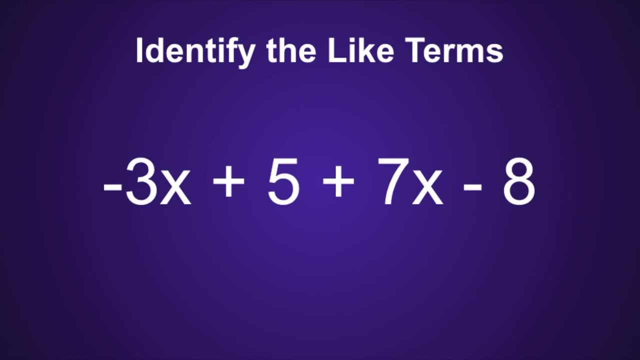 In the expression negative 3x plus 5 plus 7x minus 8,. the like terms would be negative 3x and 7x minus 8, minus 8.. I want you to press pause now. Champion, your own favorite. terms to determine silly grammar here. The same: if you arrive 4 minus 7 times, You think that the values are correct. Say minus 8 plus 9 times is also correct. You did great in your Hooke model. Now you should be pleased. you did good on the Math paper. Mm, hmm, Each of you. 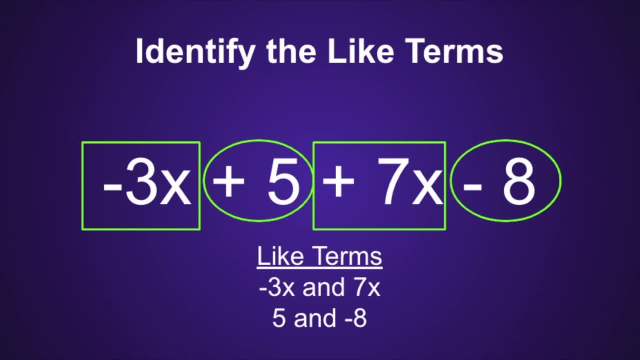 and 5 and negative 8.. Notice how I included the signs in front of the constants. For instance, instead of just positive 8, I included the minus sign so that I knew it was negative 8.. Now we're going to look at a few examples. 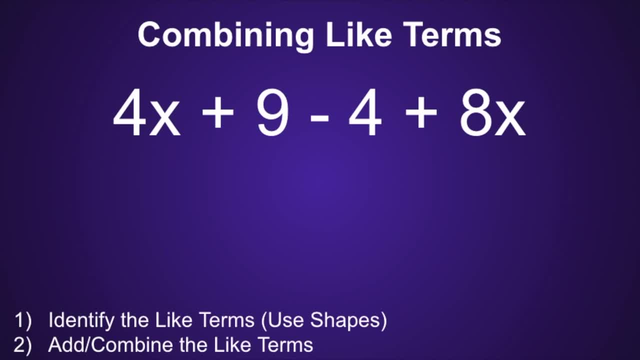 There are two steps when combining like terms. Step 1 is to identify the like terms- I like to put shapes around these so I can determine the like terms right away- And step 2 is to add or combine the like terms So in the expression. 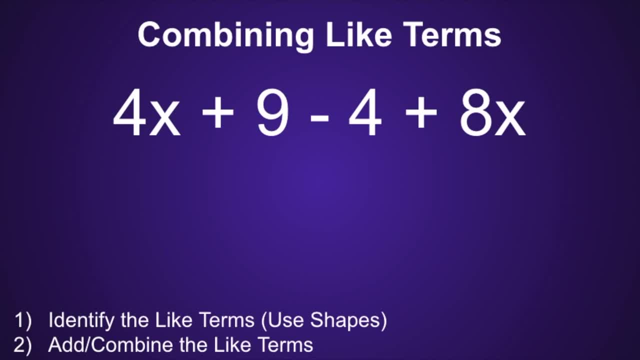 4x plus 9 minus 4 plus 8x, the like terms would be: 4x and a positive, 8x and positive, 9 and negative 4.. Now it's moving on to step 2.. Add or combine the like terms. 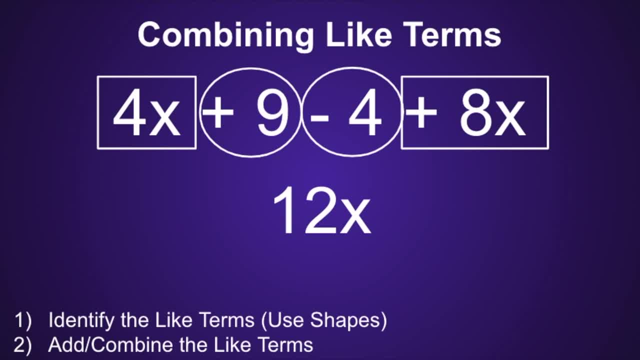 4x plus 8x is equal to 12x, And a positive 9 plus a negative 4 is equal to positive 5.. So our simplified expression would be 12x plus 5.. Here's a second example, Step 1: 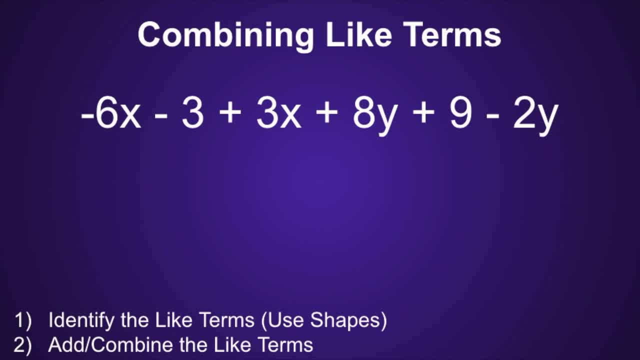 is to identify the like terms And we're going to use shapes again. The like terms in the expression negative 6x minus 3 plus 3x plus 8y plus 9 minus 2y are negative 6x and positive 3x, positive. 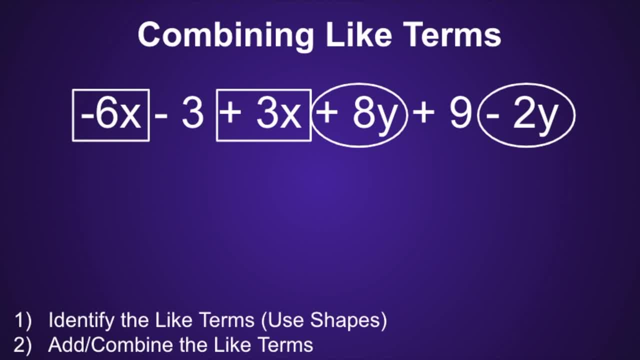 8y and negative 2y, and finally negative 3 and positive 9.. Now we can move on to step 2. Which is to add or combine the like terms. So we'll start with the x's. We have negative 6x. 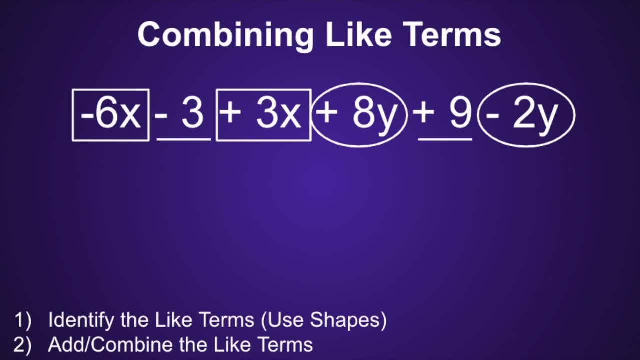 plus a positive 3x, which is equal to negative 3x. Next we'll move on to the y's. We have a positive 8y plus a negative 2y And positive 8y plus a negative 2y. 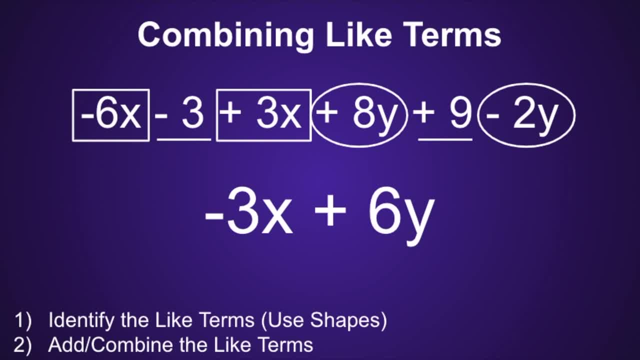 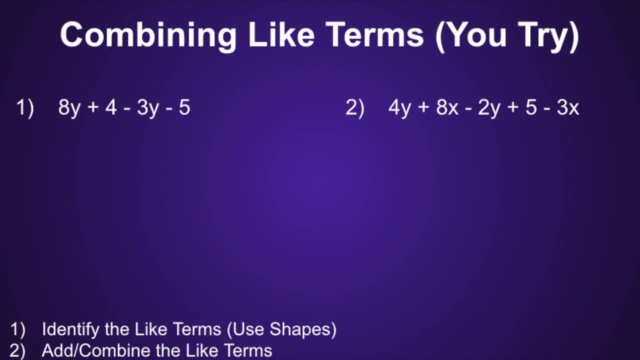 is equal to positive 6y. And finally, we have our constants, which is negative 3 plus a positive 9,, which is equal to a positive 6.. So the simplified expression would be negative 3x plus 6y plus 6.. Now I want you to try.